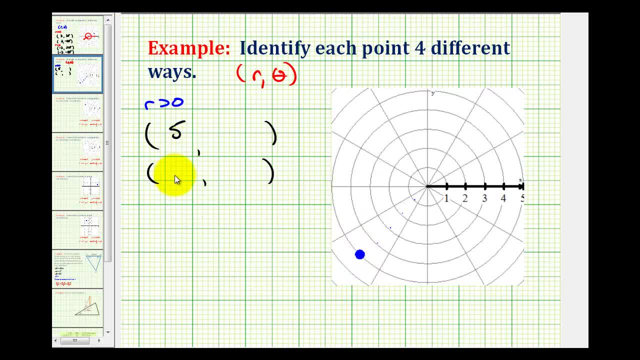 So for both of these points we'll let r equal five, And if r is positive, that means theta must be an angle in standard position where the terminal side would pass through this point, meaning the terminal side would have to be here if r is positive. 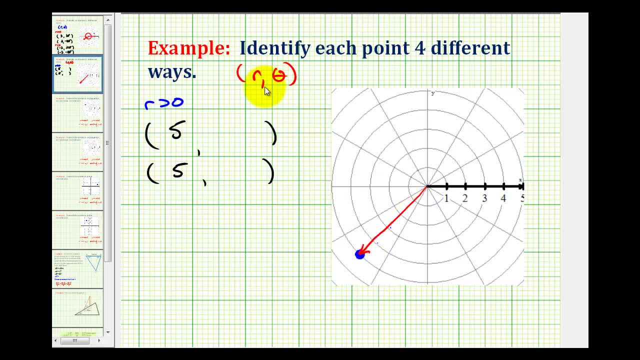 So any angle that has a terminal side here can be used for theta. So if we want theta to be the least positive angle, it would be the angle from here to here, which we could see would be 180 plus 45 degrees or 225 degrees. 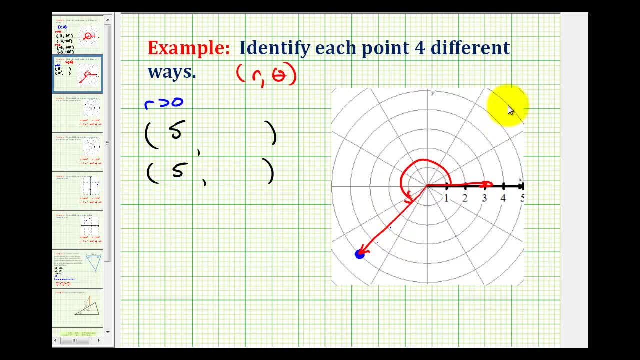 If we want to express this in radians, remember pi over four radians is equal to 45 degrees, So we could count one pi over four, two pi over four, three pi over four, four pi over four and five pi over four radians. 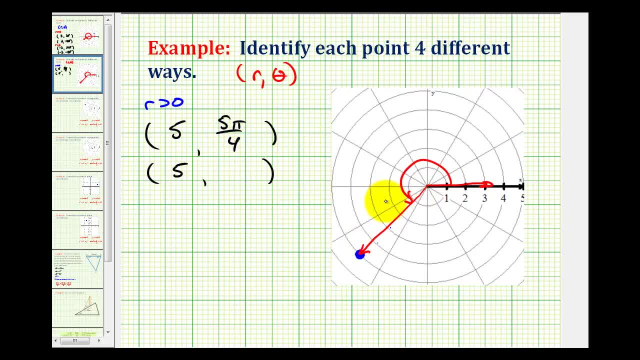 Now remember: theta can be any angle that's coterminal with this angle. So if we wanted another positive coterminal angle, we could just add multiples of two pi radians to this and we'd have another valid angle for theta. But if we want theta to be negative, the angle would have to rotate clockwise from here to here. 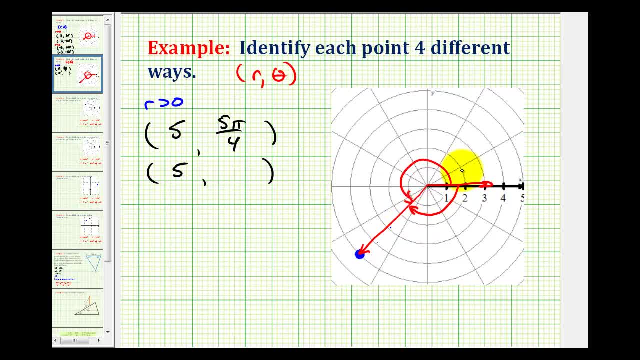 which would be negative 135 degrees, or in radians, again counting by pi over four radians, we'd have negative one pi over four radians, negative two pi over four radians and then negative three pi over four radians, And of course we could subtract multiples of two pi radians for other negative angles. 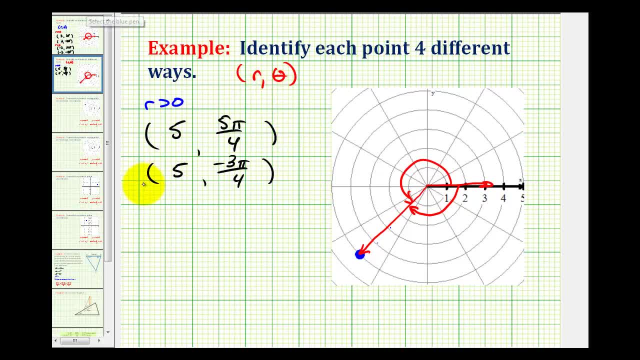 that would be correct for theta. Now let's go ahead and list two ordered pairs where r is negative or less than zero. Well, this point is still five units from the pole, so we'll let r equal negative five this time, And if r is negative or r is less than zero, then the given point lies on the ray pointing. 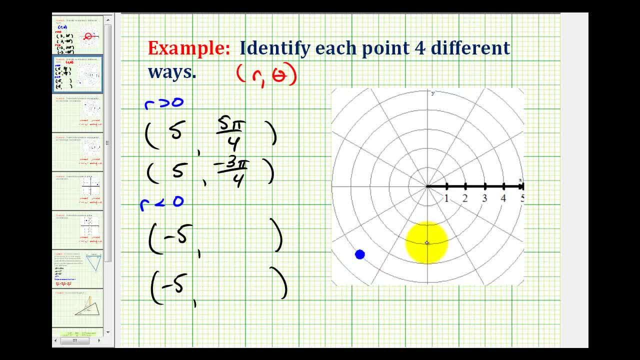 in the opposite direction of the two pi radians. So we'll let r equal negative five this time. So if r is negative, then the terminal side of theta must point in the opposite direction, meaning in this direction here. So any angle that has a terminal side in this location would be correct for theta.